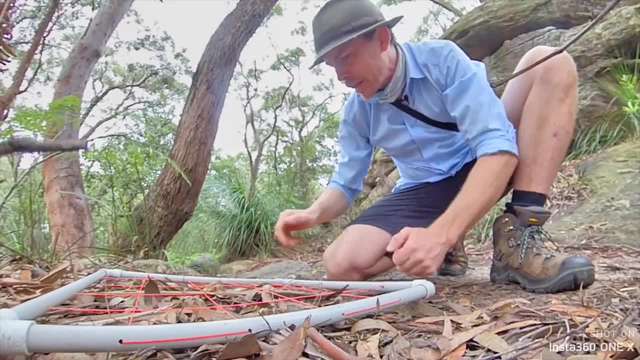 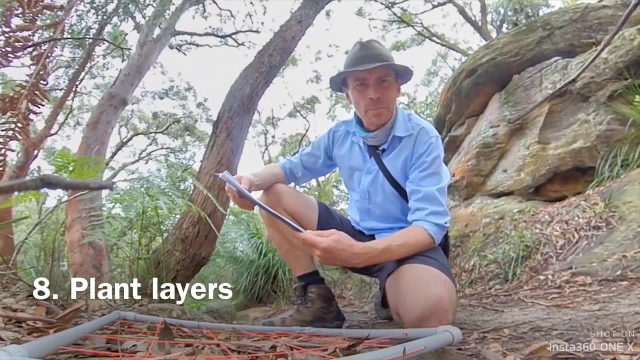 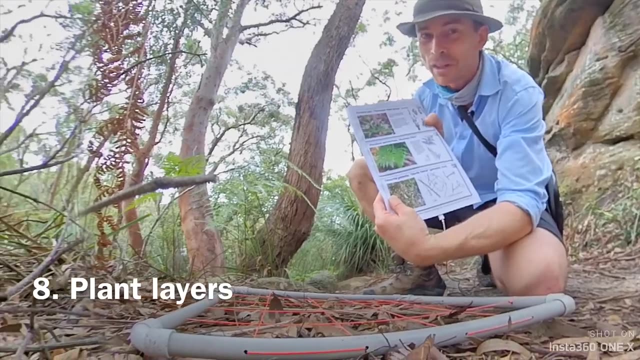 quadrat And when placed on the ground, I can estimate that we've got 90% leaf litter coverage. We can identify what sort of plants are growing here by using a plant identification key. In a forest like this, people often organise the plants into different layers Ground covers. 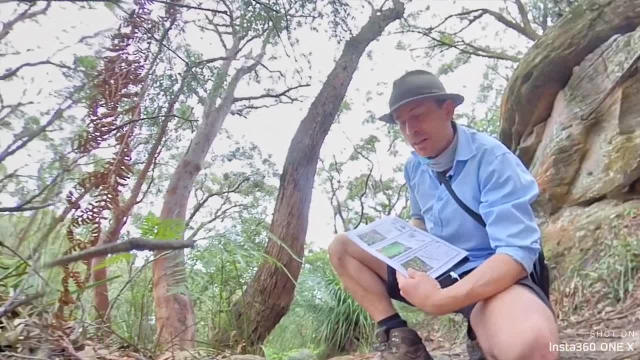 shrubs and, of course, trees. Using my key, I've identified a ground cover called Bracken fern and a tree called Sydney peppermint. Below the leaf litter, there's a tree called Bracken fern and a tree called Sydney peppermint. 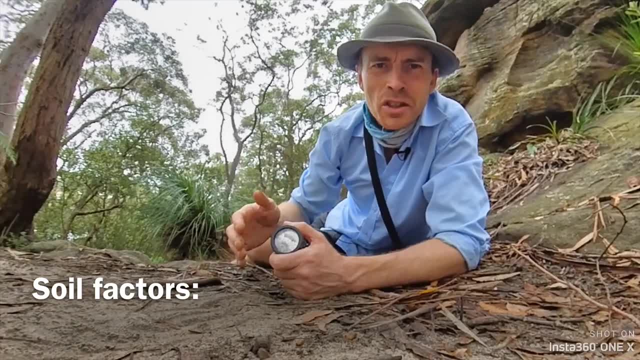 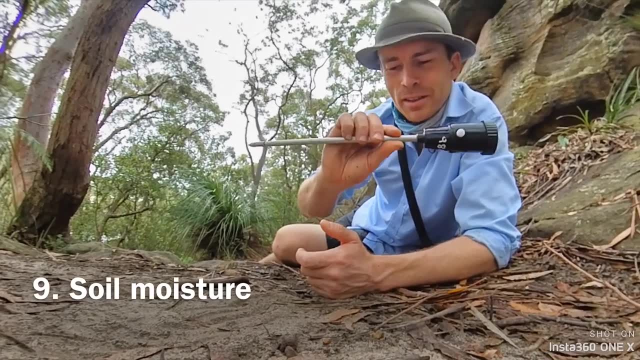 Below the leaf litter there's a tree called Bracken fern and a tree called Sydney peppermint. Soil is a mixture of rock particles, air, moisture and organic material. We can measure the soil moisture by using a moisture probe, which right now is telling me on a scale. 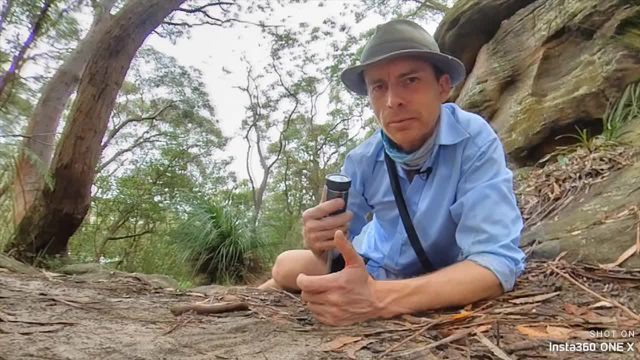 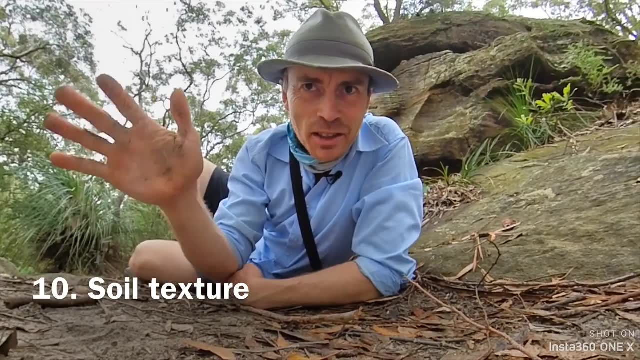 of 1 to 8, a very dry reading of 1.. Soils are not all of the same texture. Right here the soil has a sandy texture which is different to the clay soils which are often found up the top of the hills in this part. 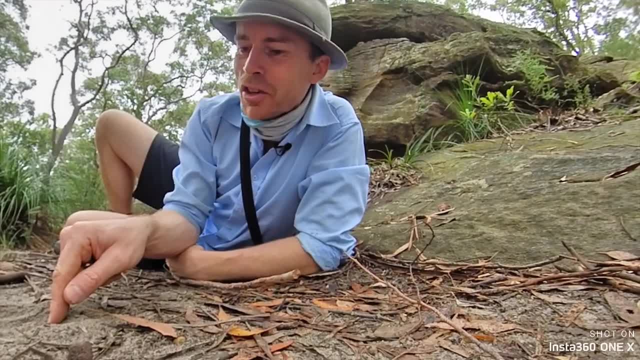 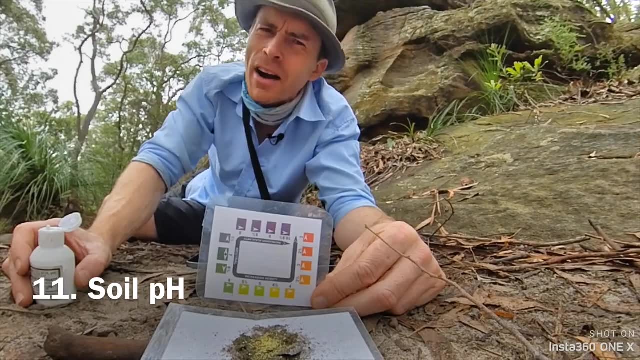 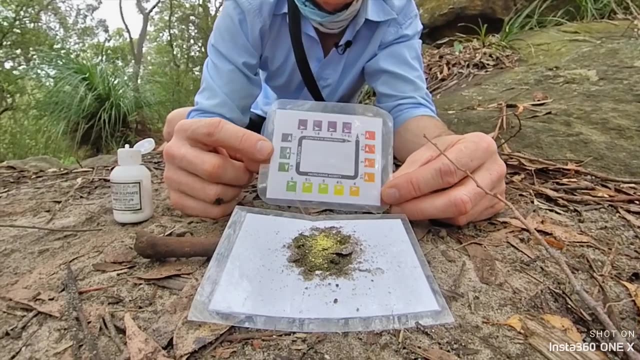 of Australia earlier. Plants and animals need different soil texture types to survive. Soils are chemically active. We can measure how acidic or alkaline a soil is by using a chemical test such as this. The barium powder has turned yellow which, according to this, 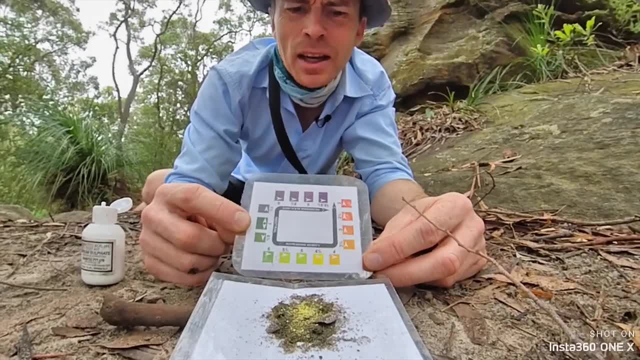 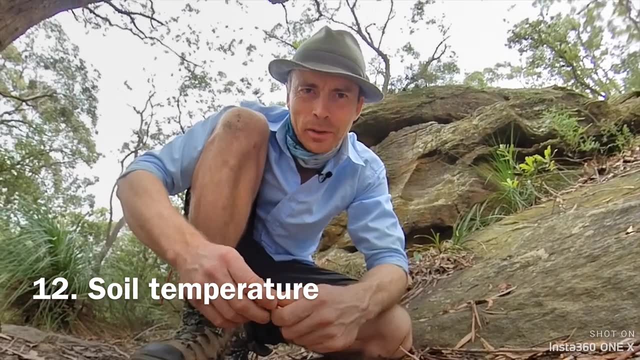 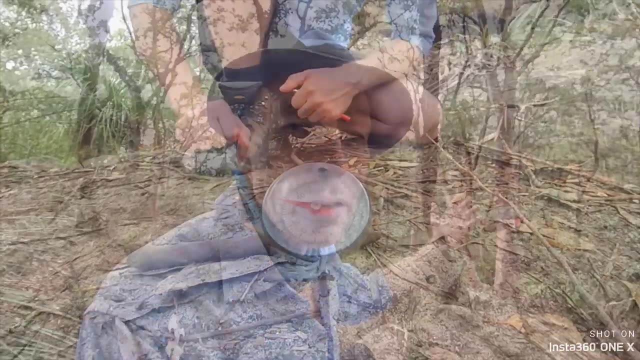 colour chart tells me that we've got a slightly acid soil with a pH of about four and a half. Soil temperature is an important factor for plant germination and growth. We can measure it using a soil temperature probe pushed into the ground like this. 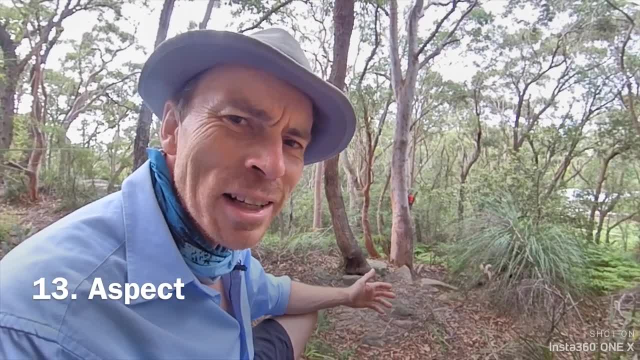 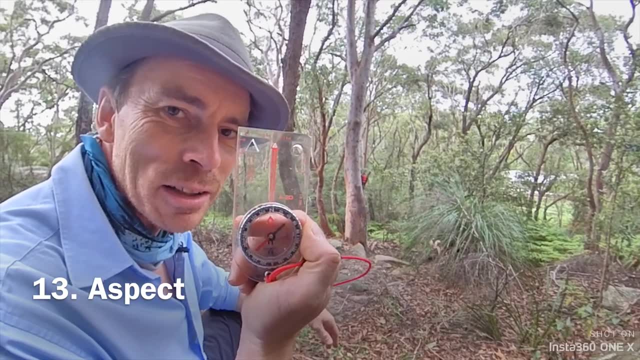 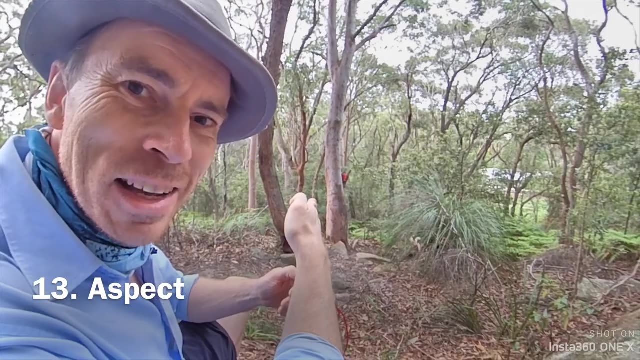 This patch of forest is on the side of a hill. The direction the slope of that hill faces is called its aspect. We can record the aspect using a compass like this. So let's see North's behind me South's. that way, In this case, the hill has a south-easterly aspect. 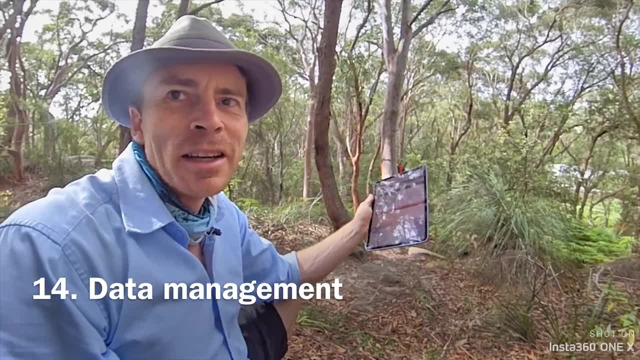 I've been collecting all this information in a data table on my iPad. I've been collecting all this information in a data table on my iPad. I've been collecting all this information in a data table on my iPad. Now I can use the information as data to compare with other places, Or maybe I can plan to.